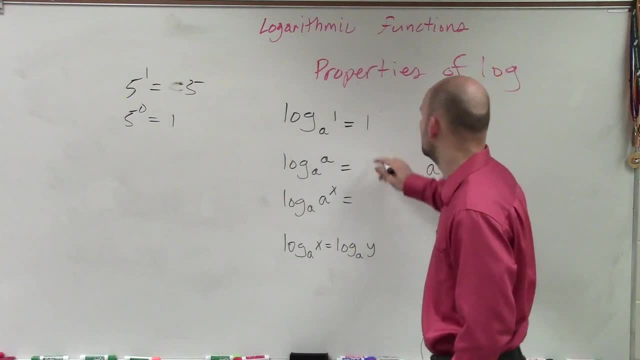 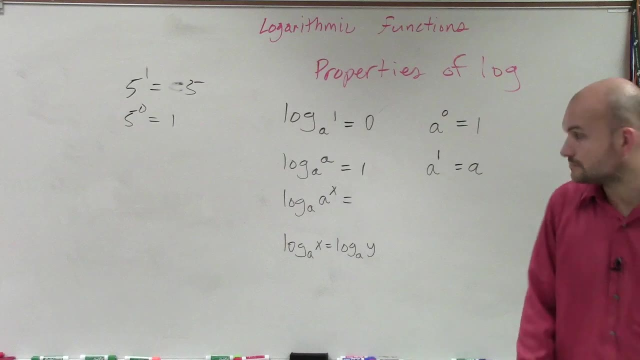 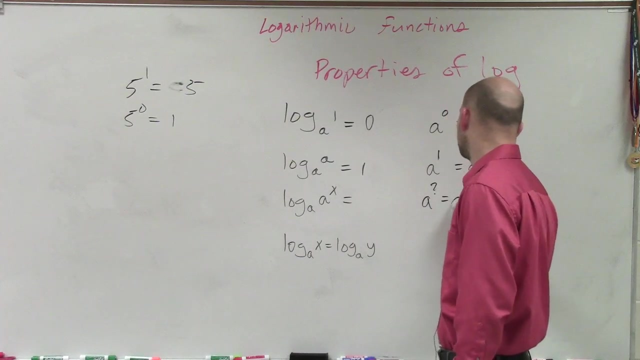 Oh, Yeah, yeah, yeah, I'm sorry, That's supposed to be 0.. Sorry, I just wrote it wrong. Thank you, Yes, you are correct. The next one. So log base a of x. So now I've got to say a raised to what power equals a to the x. 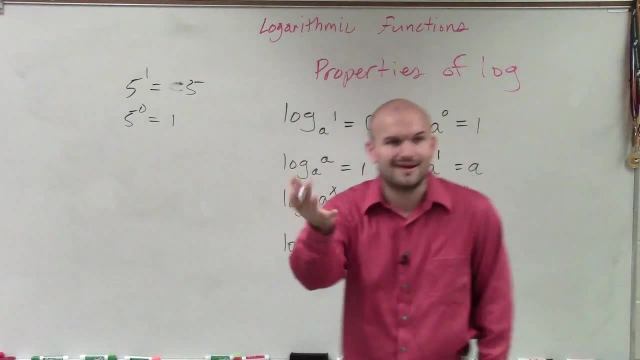 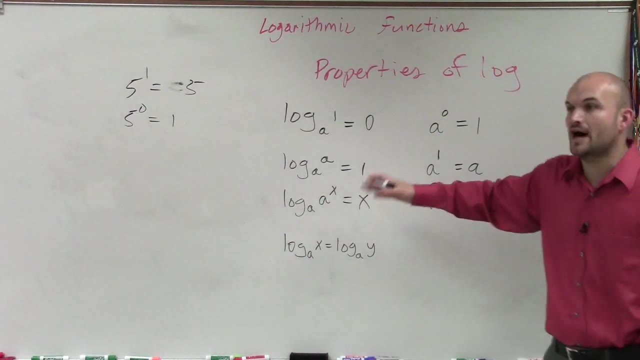 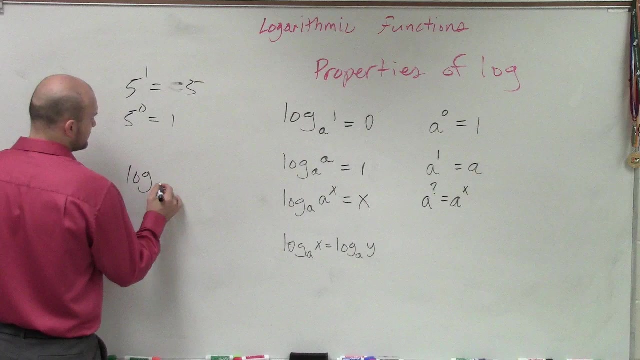 So what does that power have to be, That question mark, What does that have to be x, x, right? So a lot of times what we say, if you guys have log base a of a raised to the x, that just equals x. So just a quick little example: if I said log base 5 of 5 squared, 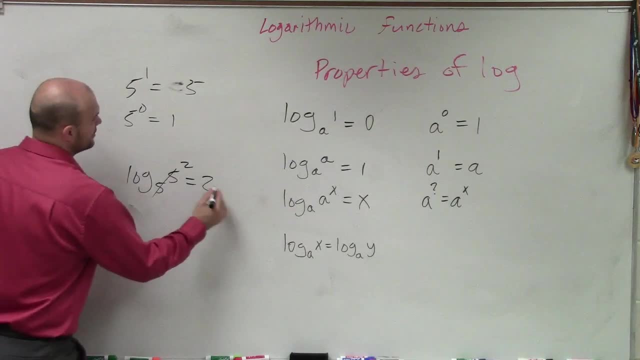 well, you guys can just write those out And you're going to get a log base, a of a raised to the x to write those out and just say that's going to equal 2.. Yes, And that can be canceled out. It doesn't really cancel out. 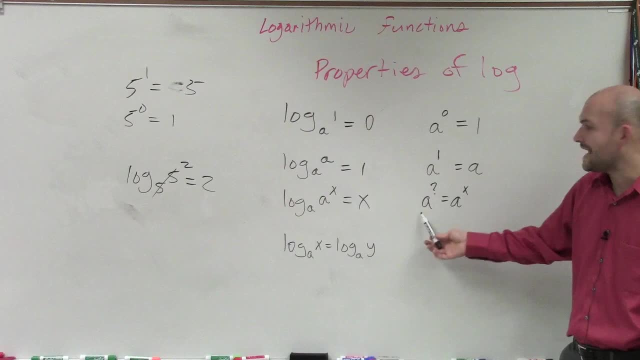 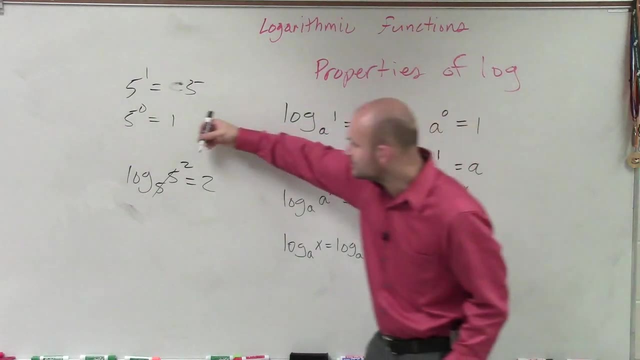 But what you can say is because, look, if I rewrite this in exponential form: a raised to what power equals a to the x? That question has to be x, right? So therefore you can just say: you just take when I have a logarithm with the base raised. 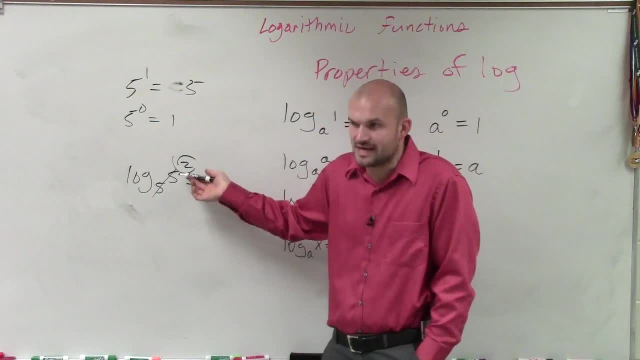 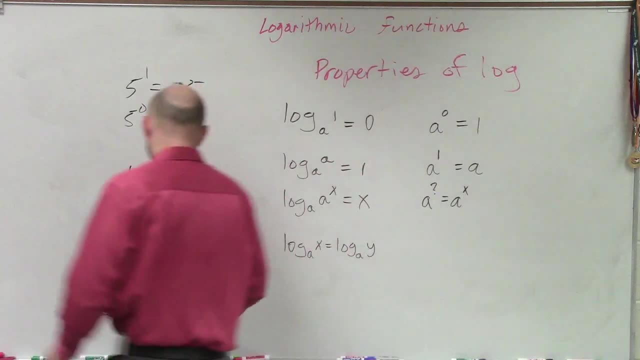 to the same base of an exponent, it just equals the exponent. No, Do you guys understand this? OK, so watch. If I say log base: 5 of 5 squared, what does that equal? So therefore, that is, 5 raised to the x power equals 5 squared. 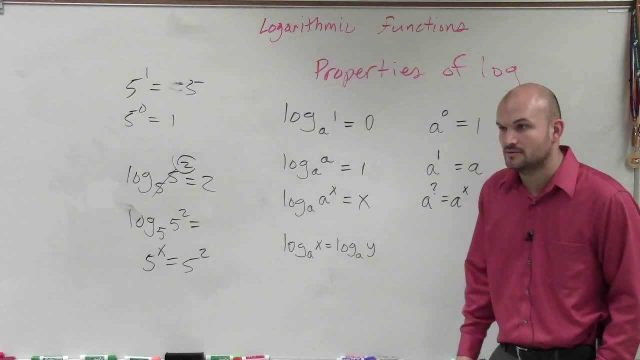 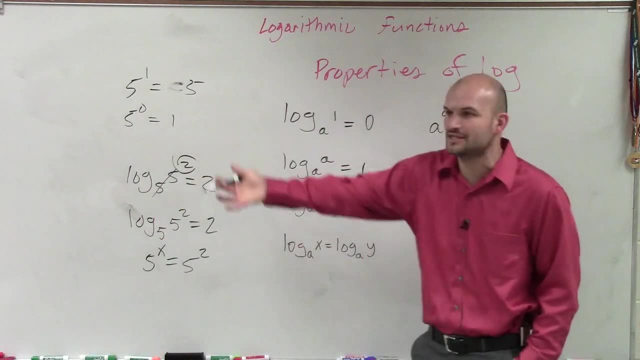 So what does you have to raise 5 to to get to be 5 squared 2.? So I know I put a line through them, but they're not really canceling each other out, They're just you apply, Then I'm just using those rules. 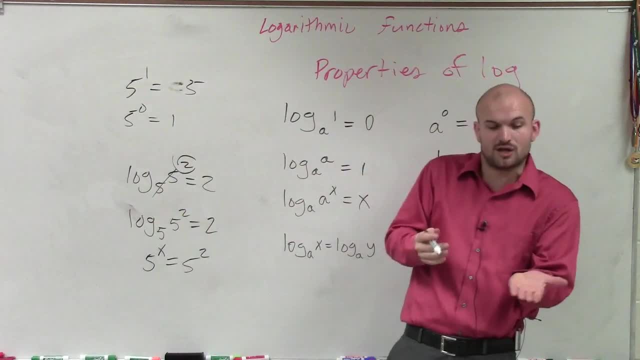 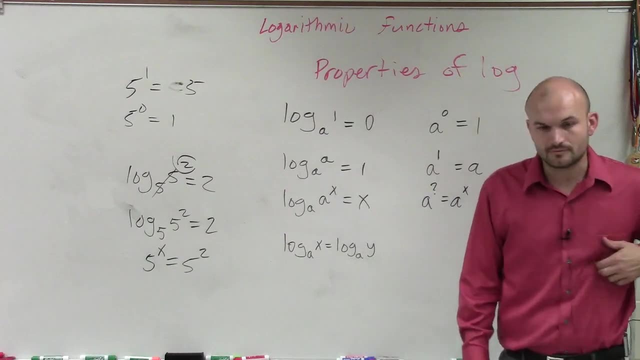 But yes, if you just want to think about it, just take that exponent. As long as you have the same base of a logarithm, evaluate it for the same base of an exponential, then yes, you can just take the exponent, OK. 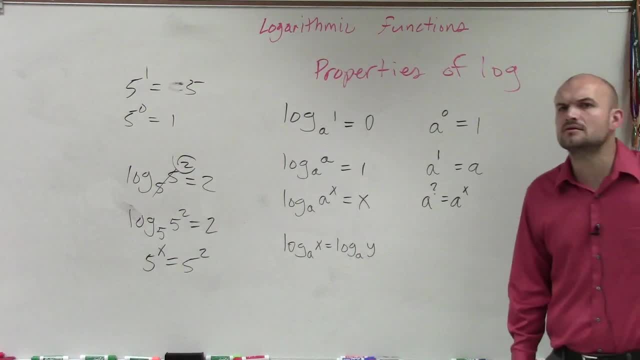 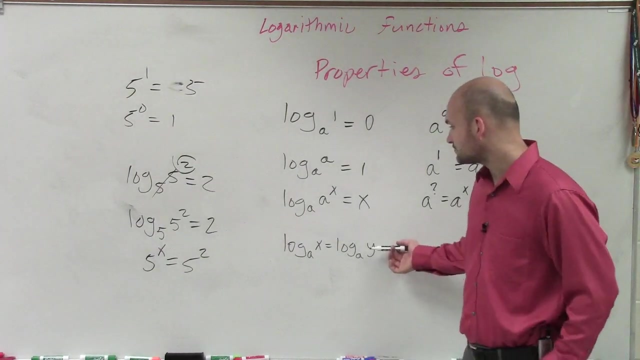 Last one: log base a of x. Yes, No problem. Now the last one. if I have log base a of x equals log base a of y. if you have the exact same base of something, the exact same base, then what you can have is you can just: